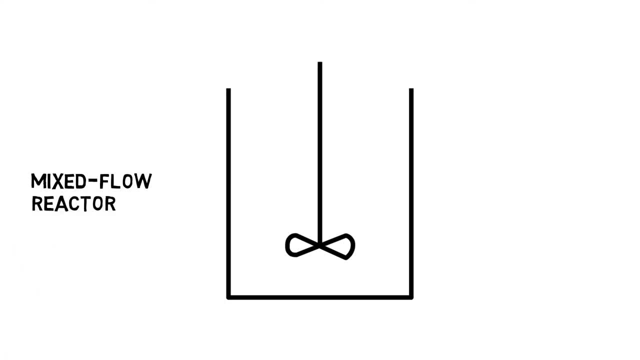 That is, a reactor which is fed continuously with a mixture of raw materials and with the continuous removal of the reaction products. Unfortunately, some molecules of the raw material have a very short residence time inside the reactor, Others spend a slightly longer time in the reactor before exiting, and yet others have an extremely long residence time In 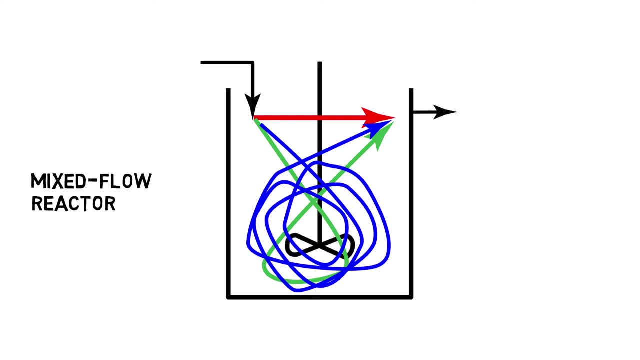 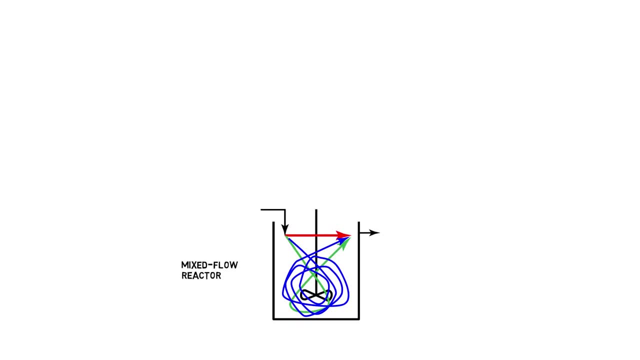 fact, in a continuous stirred tank reactor, or CSDR, the number of possible residence times is infinite. To illustrate this, one can draw a graph of the reactor With the different possible residence times in the CSDR along the x-axis and their probability. 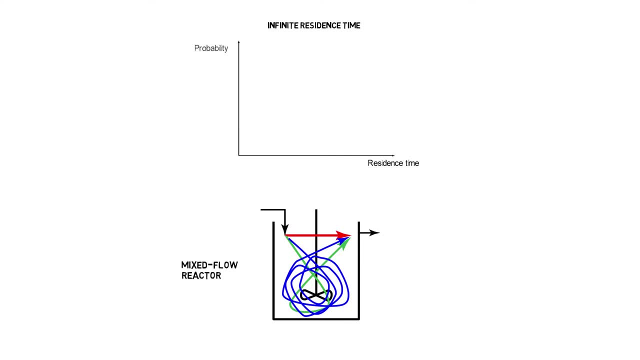 to occur on the y-axis. In other words, this graph shows the number of molecules exiting the reactor at each of the different times. It can be seen that there is a large number of molecules with a short residence time, a few number of molecules with a very long 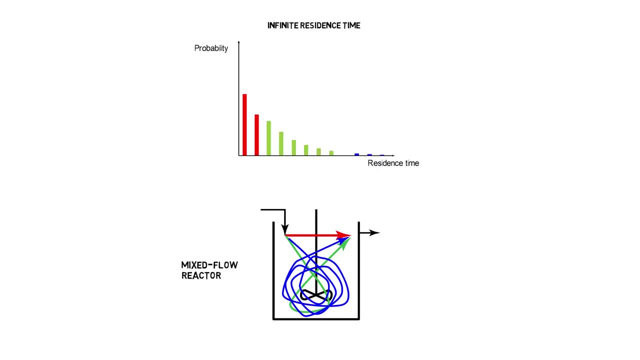 residence time and many molecules with residence times in between both extremes. The result of this graph is that the number of molecules exiting the reactor at each of the different times is infinite. The resulting curve has the shape of a decreasing exponential function. Let's return to the industrial scale stirred tank reactor. Another problem is that the 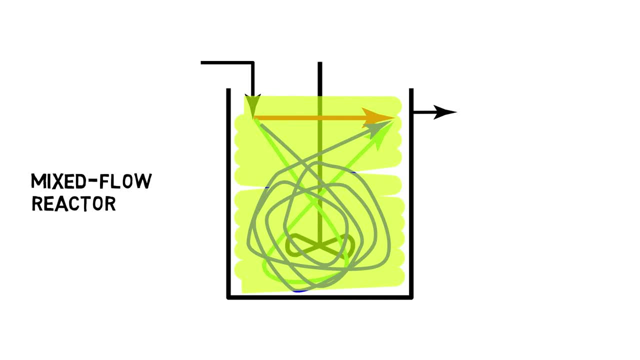 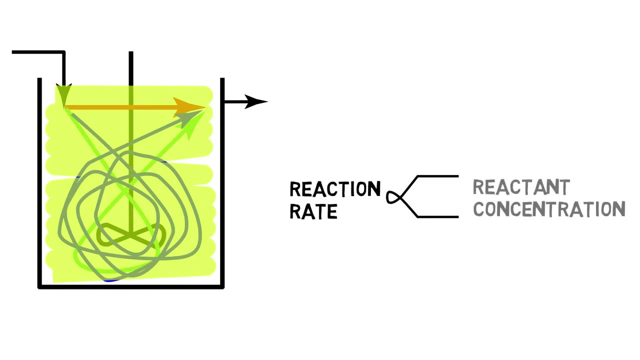 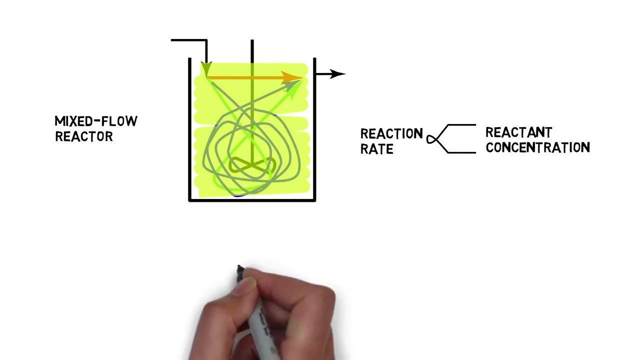 concentration of the reactant is uniform throughout the reactor, since the reactor is stirred continuously and this concentration is low because it corresponds to the concentration at the outlet of the reactor. However, the reaction rate is usually proportional to the reactant concentration. Hence, in a stirred tank reactor, the reaction rate is low throughout the entire volume of. 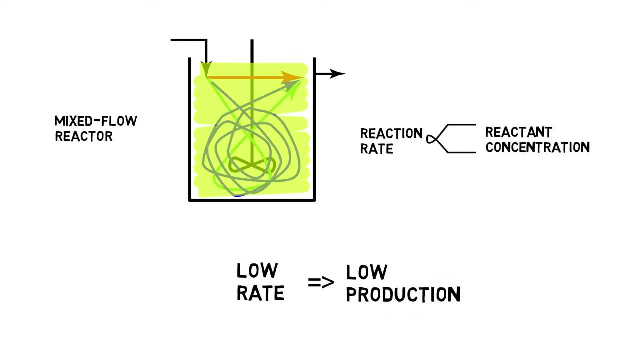 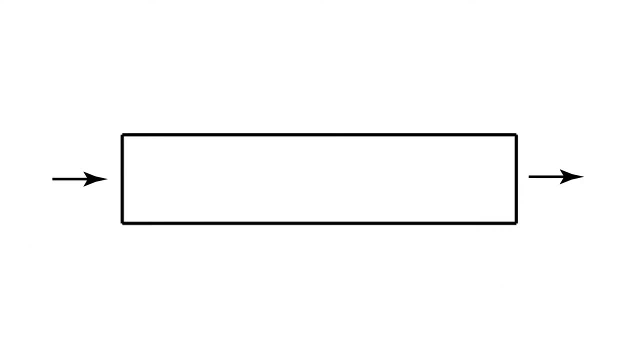 the reactor, and this results in a low production of the molecule of interest. In order to overcome this, we can design a reactor without a stirrer, so that zones with different degrees of concentration exist. The reactant concentration will remain low close to the reactor outlet, but it will increase as you move towards the reactor inlet and 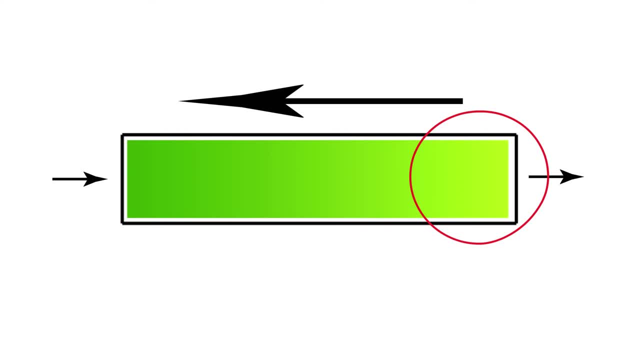 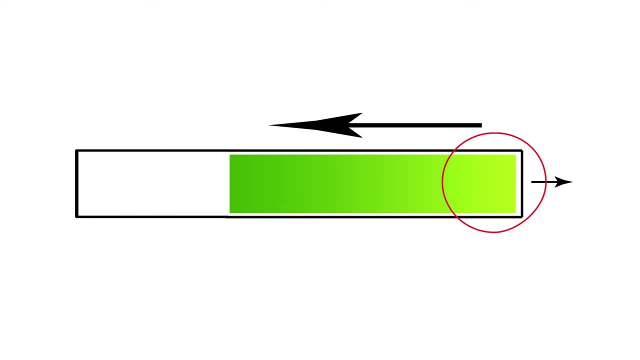 therefore, the reaction rate will also increase towards the inlet. In addition, if the length of the reactor is increased, the residence time of the reactive molecules will also increase, giving them time to be transformed into the desired molecule. This was how the tubular reactor was invented. The corresponding ideal reactor is generally: 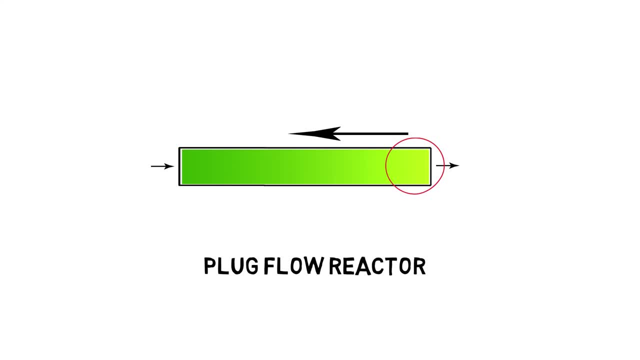 called a plug-flow reactor. So what is the explanation? In a plug-flow reactor, all the molecules move through it at roughly the same speed. You can imagine a piston that moves forward inside the reactor at a constant speed, pushing the fluid. The molecules that are located in a small section of this reactor are hardly 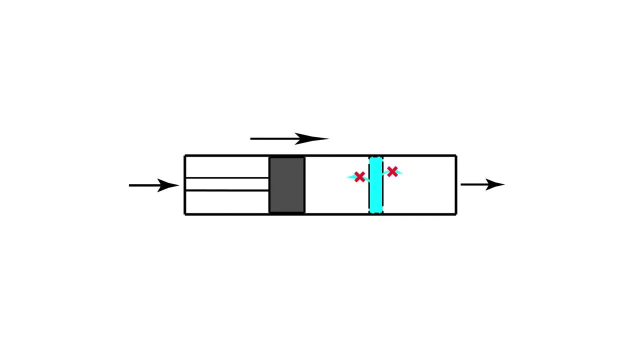 mixed with the molecules just behind them or just in front of them. This type of behaviour does not actually exist in reality, but we can get quite close to it. The plug-flow reactor is an ideal reactor which is used as a guideline for the design of industrial tubular reactors. 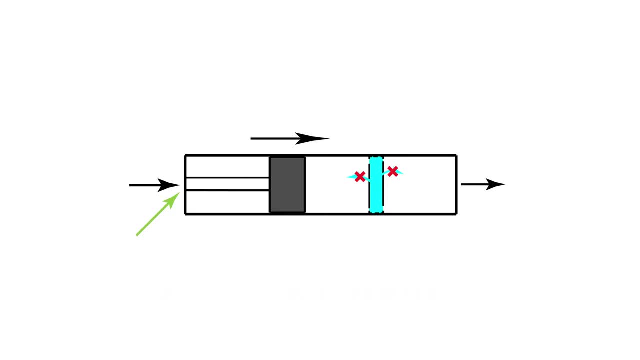 Let's imagine the injection of a non-reactive tracer at the inlet of the reactor in the form of a pulse input, which means that the amount of tracer is injected instantaneously. If a probe is placed at the outlet of the reactor, we will be able to follow tracer. 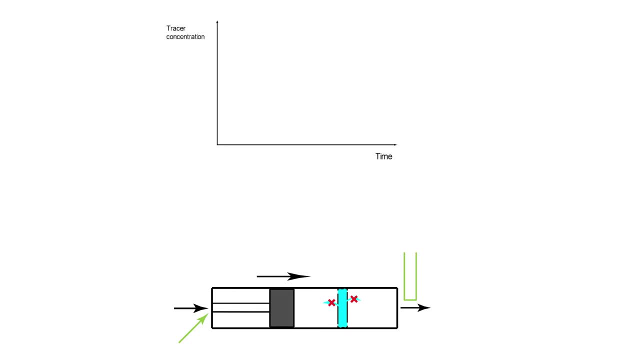 concentration at the outlet as a function of time. If the reactor is a perfect plug-flow reactor, the exit time of the reactor will be the same as the exit time of the reactor. The exit signal will have this shape. We can see the pulse input corresponding to the. 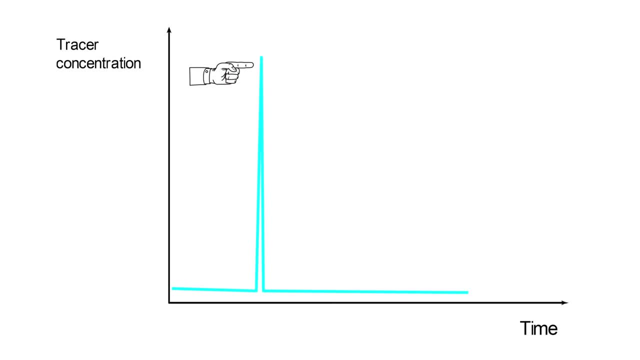 injection of the tracer, which is just shifted in time. All of the molecules have the same residence time, which is the time measured between the injection of the tracer and the peak observed at the exit. We can understand intuitively that this time also corresponds. 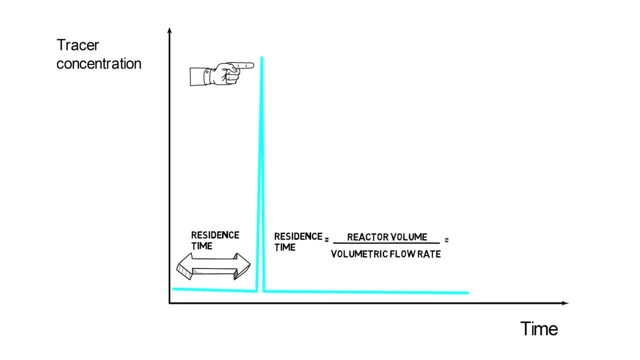 to the ratio between the reactor volume and the volumetric flow rate. This is also called the space time In a CSDR. on the other hand, the residence time distribution decreases exponentially with time. A large amount of tracer exits the reactor after a. 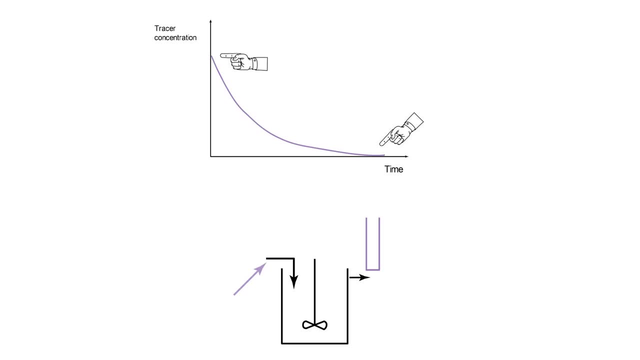 short time, after which less and less tracer is detected at the outlet. However, this wide distribution of residence times in the CSDR has an adverse effect on the production of the desired molecule. In fact, it is preferable to use a reactor in 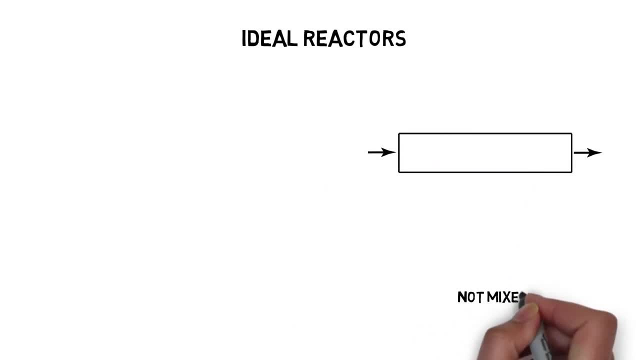 which the residence time distribution decreases exponentially with time. This is also called the time distribution of the reactor volume. In the CSDR the residence time distribution is narrow. That is where all the molecules exit the reactor at the same time, like in the plug flow reactor- Sometimes a plug.